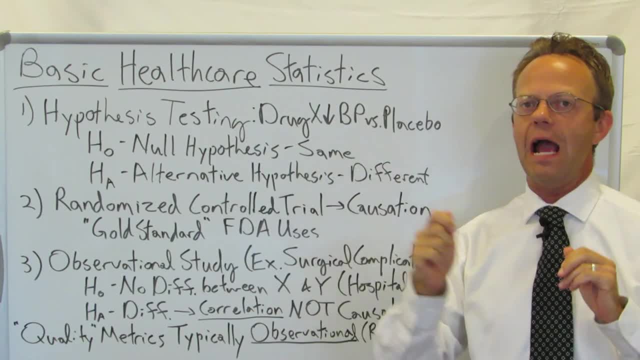 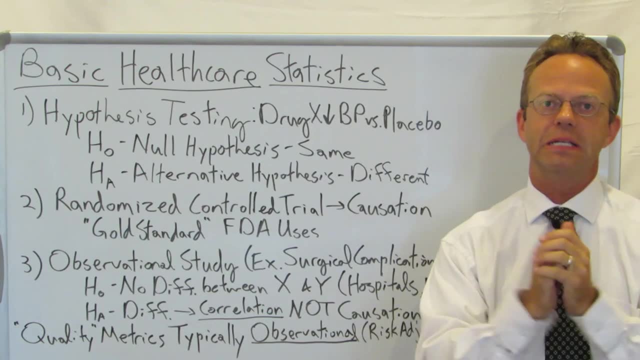 you are sticking with me, So thank you so much for that. So, for today, I promise to make it very short and very practical. Okay, but we're dealing with data- a lot in health care, and so we have to have a basic understanding of statistics. So when data analysis is performed, 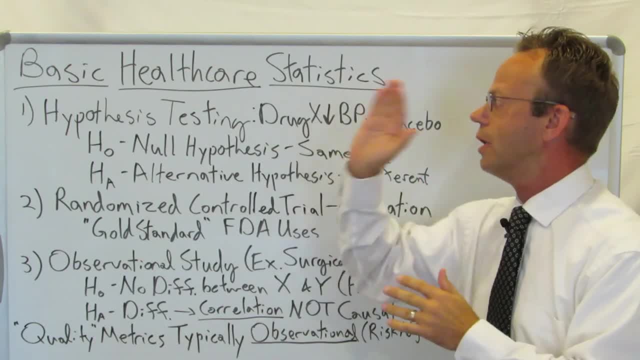 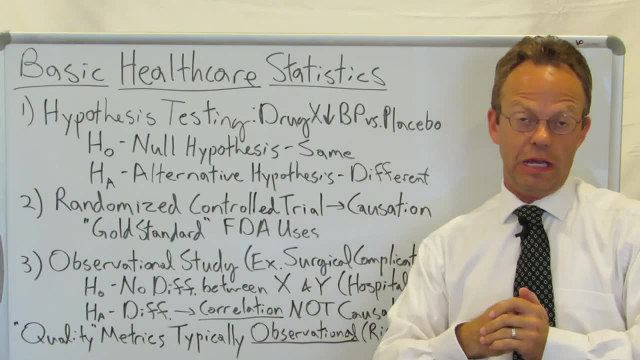 sort of the basic level of understanding that we all need to have is something that's called hypothesis testing, and it's typically used in, like, let's say, a drug trial, but it's used essentially all over the place when you're dealing with statistical analysis. But let's 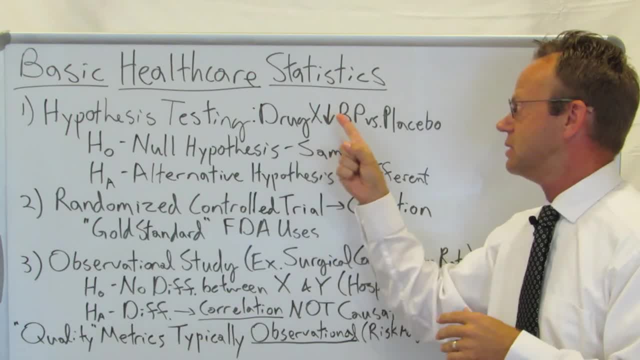 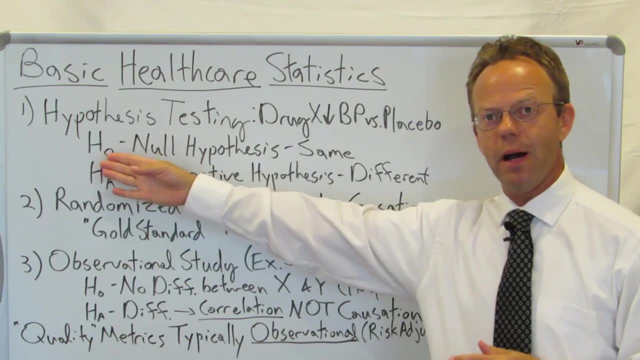 just use the drug trial example, where you have drug X. let's say, does it lower blood pressure versus placebo? Now you have two hypotheses. You have what's called the null hypothesis, You have the no hypothesis and you have the no hypothesis And you have: 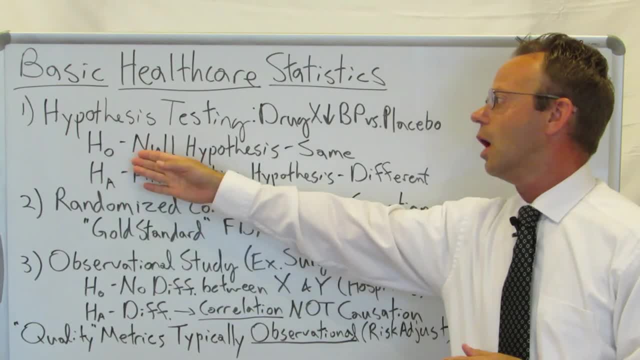 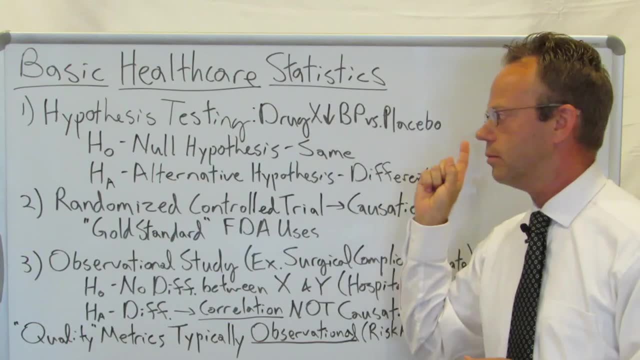 the no hypothesis, which is abbreviated H naught, or H with a little sub zero, which is the null hypothesis, which means there is no difference between the tested blood pressure drug and placebo, sugar pill, et cetera. Okay, and then there's the alternative. 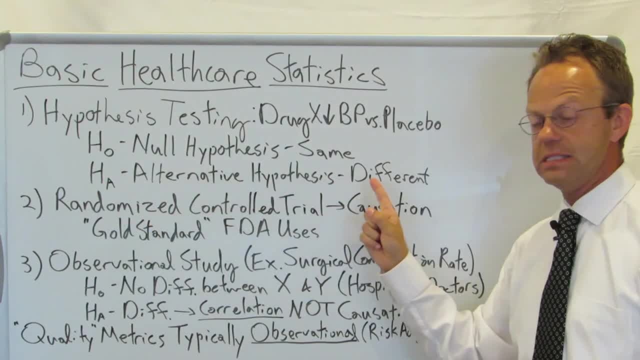 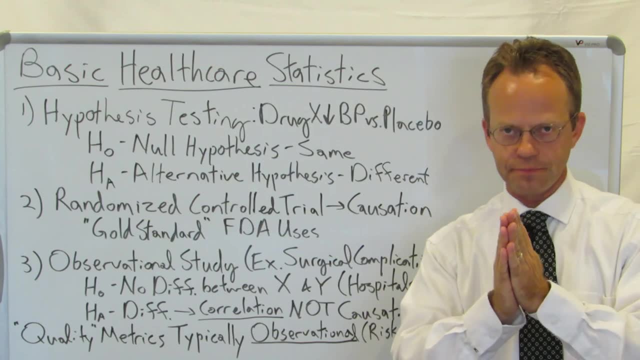 hypothesis, which is abbreviated H sub A, and that is is that they're different. Okay, so what you're doing with hypothesis testing is you're looking at their data and you're saying, hey, is there a difference? And that's important, because notice that you have to. 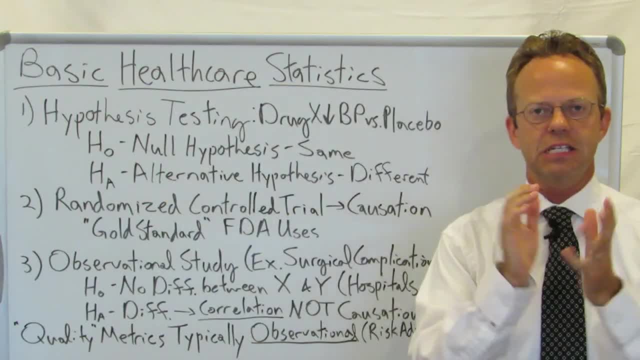 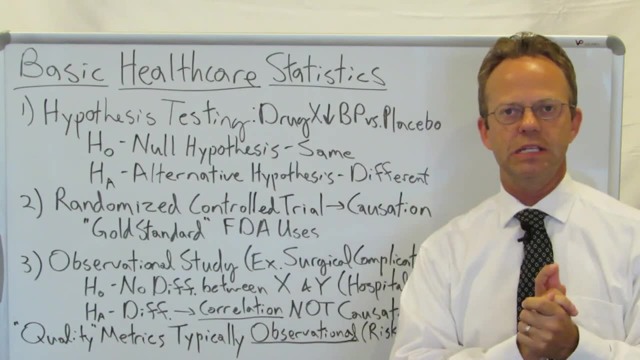 form, a specific question or a hypothesis, And you're looking at the data and you're looking at the hypothesis that you're testing when you're looking at the data. Okay, well, there's different ways to generate data and we're only going to do two of those ways today. 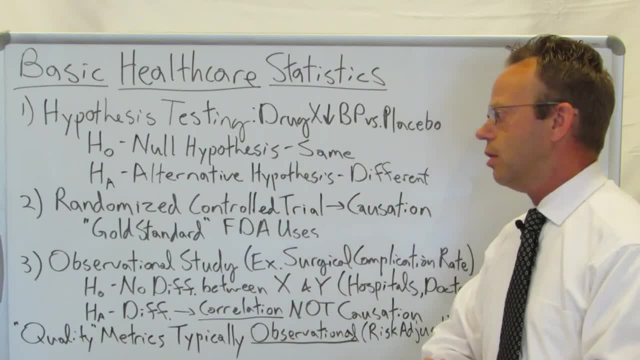 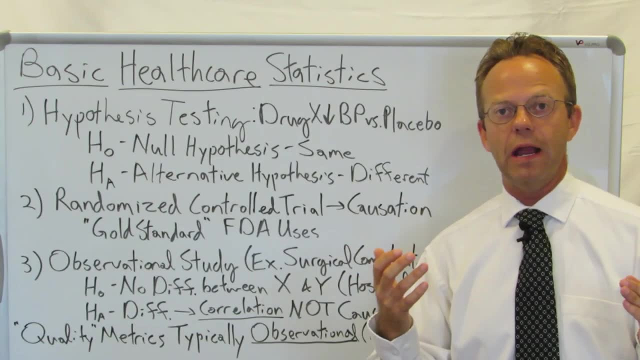 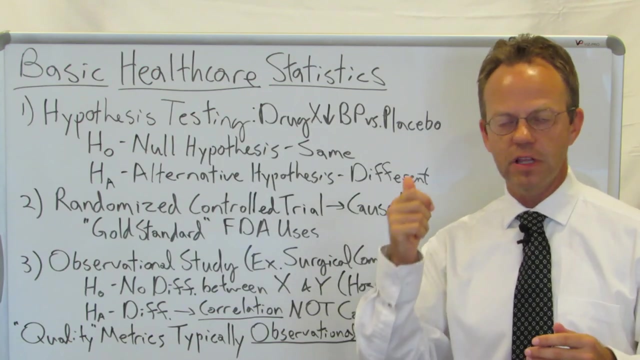 And related to the drug trial. we have what are referred to as randomized controlled trials. So this is sort of the gold standard. This is what the FDA uses where one it's randomized. So in this situation here, if you have a group of 100 people, then you're going to flip a. 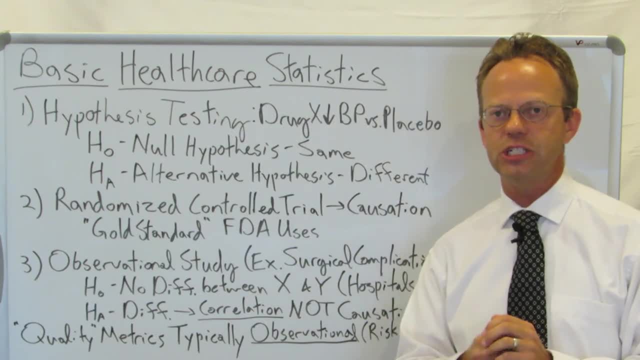 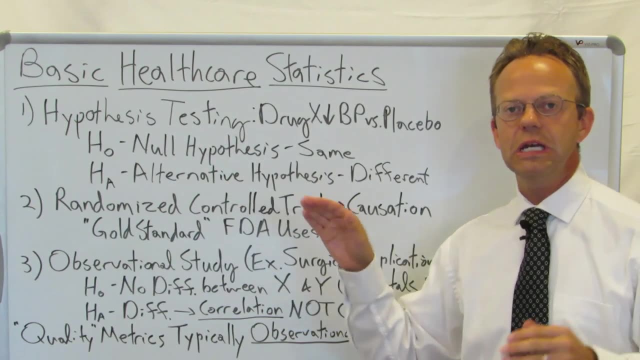 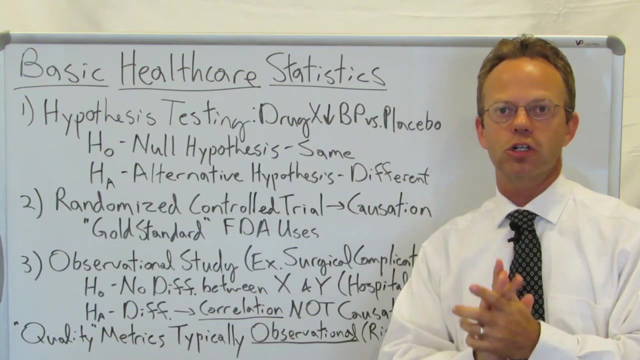 coin and say: heads, you get the Blood pressure medication, tails, you get the placebo. Okay, so it's randomized And then it's controlled, in that all the other situations around the person's blood pressure are controlled as much as possible, And the reason for that is because you're testing. 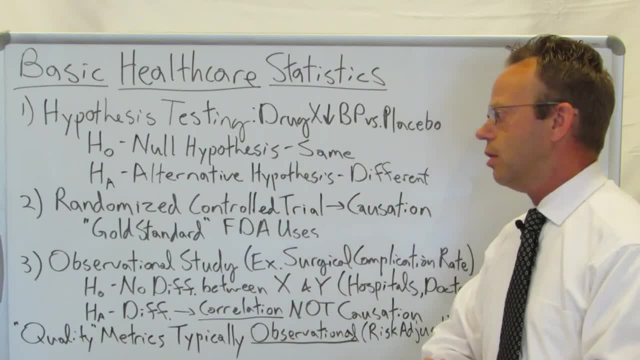 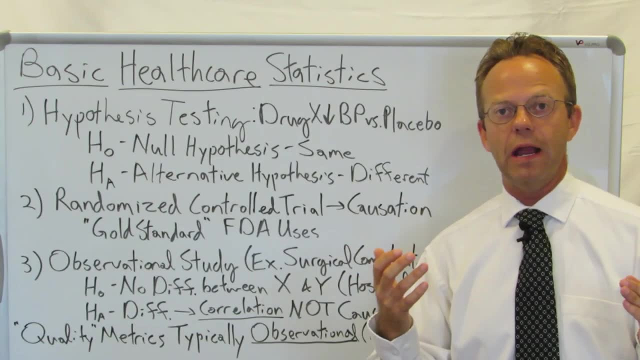 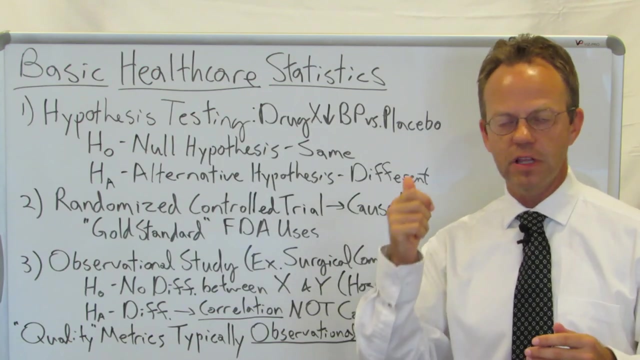 And related to the drug trial. we have what are referred to as randomized controlled trials. So this is sort of the gold standard. This is what the FDA uses where one it's randomized. So in this situation here, if you have a group of 100 people, then you're going to flip a. 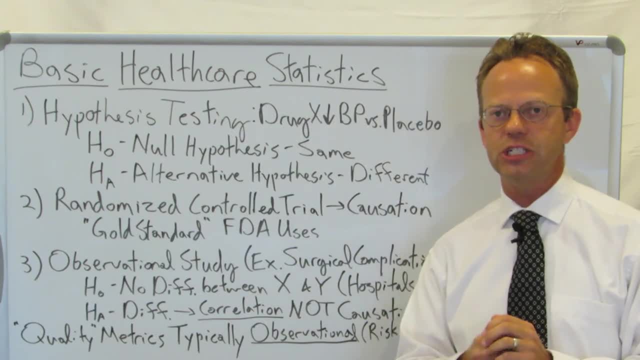 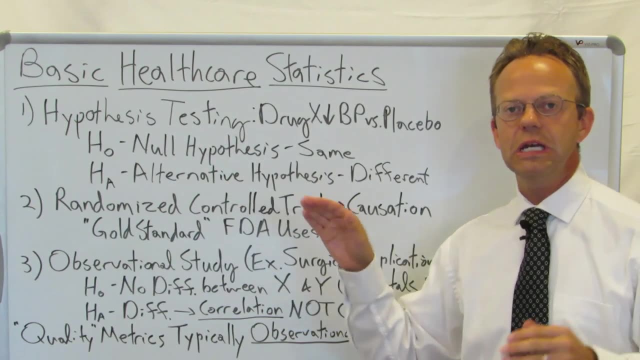 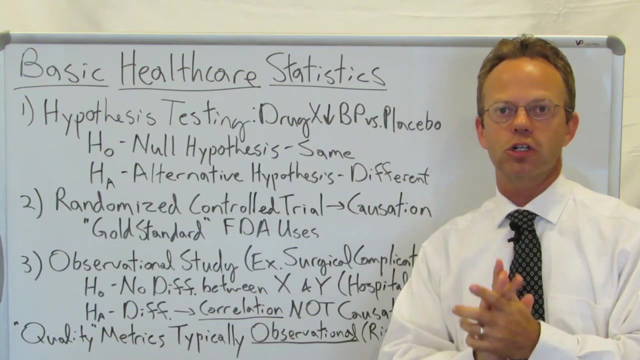 coin and say: heads, you get the Blood pressure medication, tails, you get the placebo. Okay, so it's randomized And then it's controlled, in that all the other situations around the person's blood pressure are controlled as much as possible, And the reason for that is because you're testing. 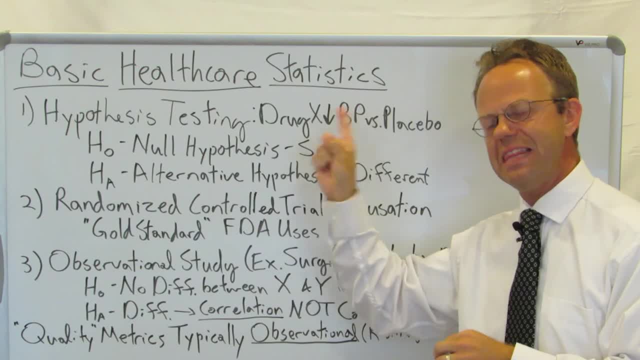 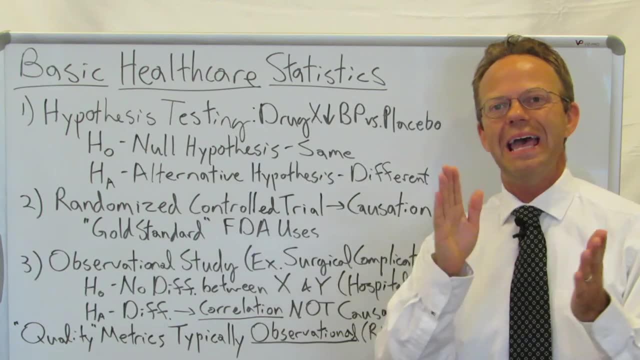 specifically this intervention to see if this specific thing here is what's causing the change in the blood pressure as opposed to something else. Okay, and that has to be done on a prospective basis. And not only do they do that, but they also oftentimes double blind it, meaning that the 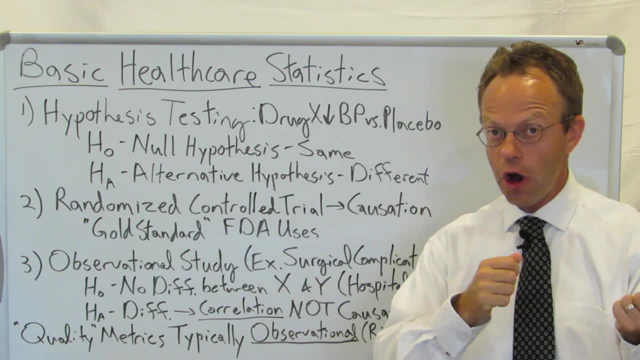 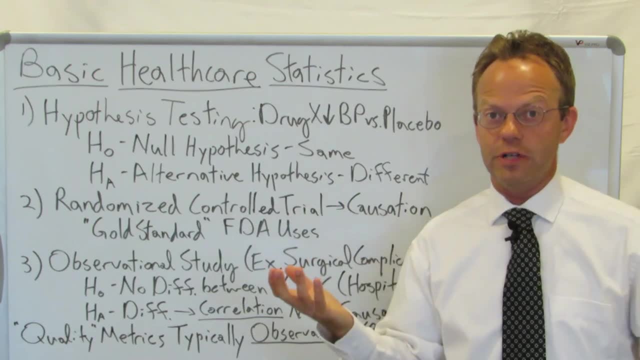 patient or the test subject themselves doesn't know whether they're taking the blood pressure pill or they're taking the placebo. Because, let's say, you take the placebo and you know you're taking the placebo, and you're all stressed out that you're taking the placebo because you're. 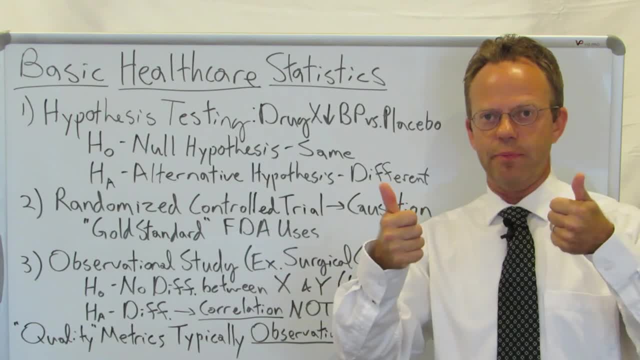 like: oh, that's not going to work, It's only a sugar pill, And so that raises your blood pressure. And so you might say: oh well, look, the blood pressure pill works versus the placebo, because the people taking the placebo were stressed. 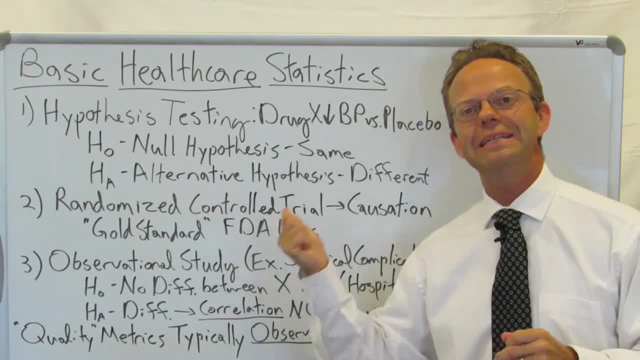 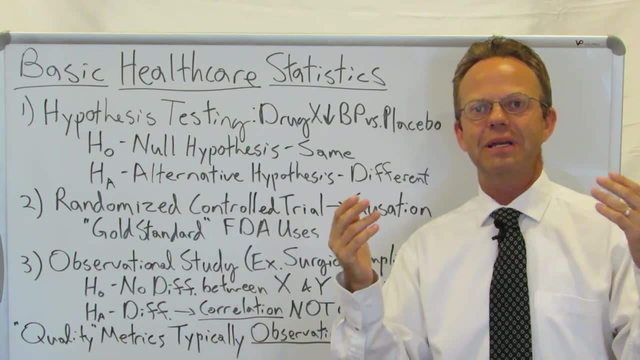 Okay, so that's why it has to be blinded. And then it even has to be blinded to the researchers themselves When they're analyzing the data. they can't know which group had the placebo versus the blood pressure pill, because the researchers themselves will subconsciously 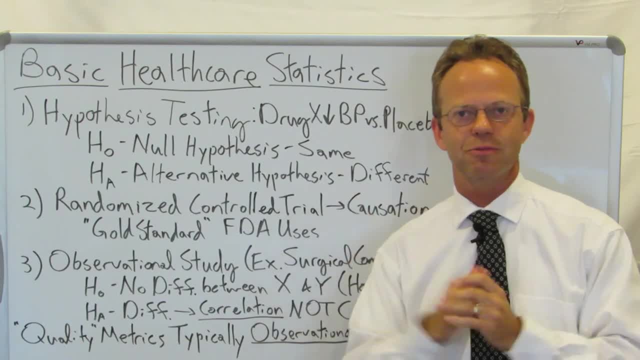 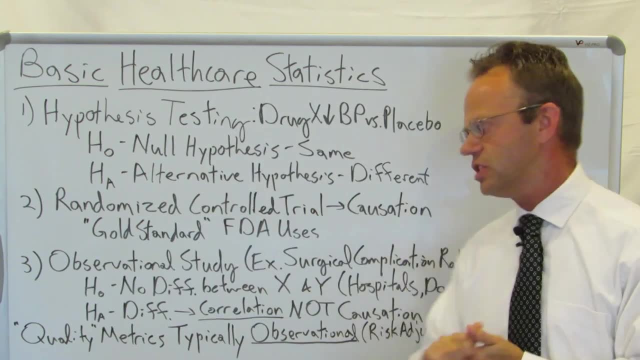 or consciously bias their analysis of the data to give them the results they want. Okay, fine, What's another way to generate data? It's referred to as an observational study, right, And so this is where you know we might observe a surgical complication rate. 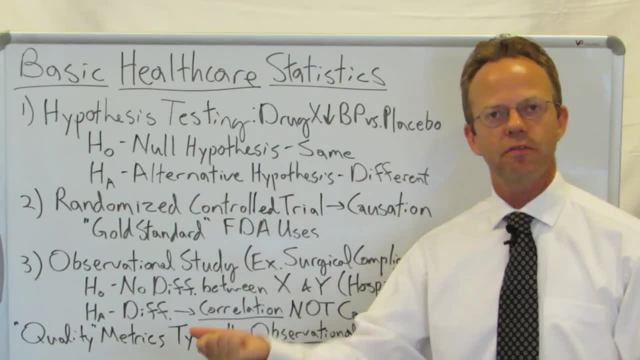 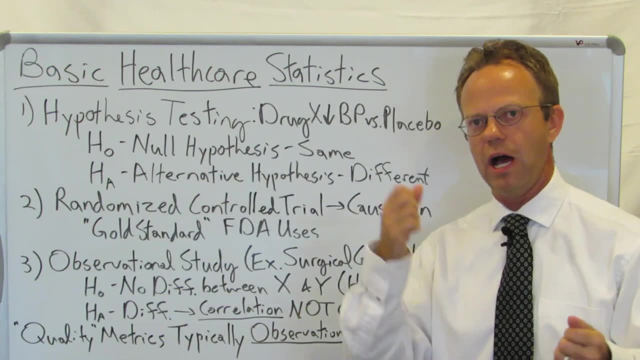 at one hospital. Okay, so this is where you might observe a surgical complication rate at one hospital versus another, or for one surgeon versus another. Again, you can have a null hypothesis which says there's no difference between X and Y, no difference between one hospital or another, no difference between 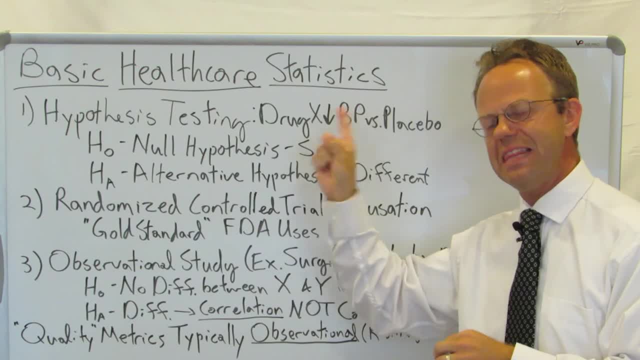 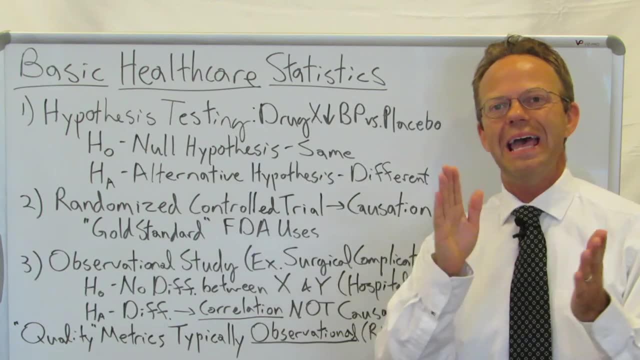 specifically this intervention to see if this specific thing here is what's causing the change in the blood pressure as opposed to something else. Okay, and that has to be done on a prospective basis. And not only do they do that, but they also oftentimes double blind it, meaning that the 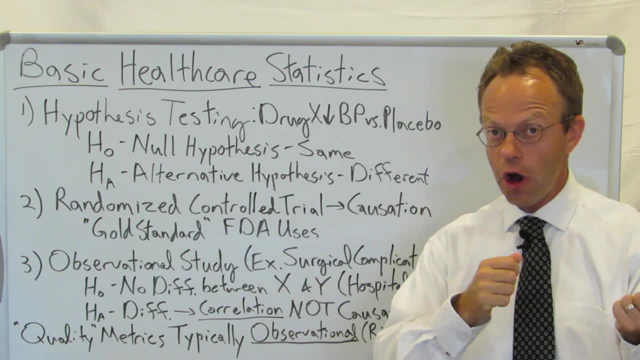 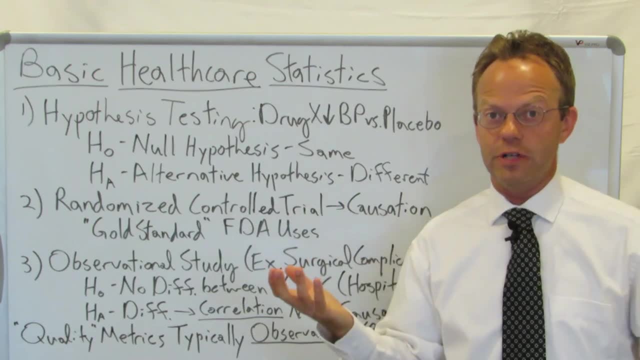 patient or the test subject themselves doesn't know whether they're taking the blood pressure pill or they're taking the placebo. Because, let's say, you take the placebo and you know you're taking the placebo, and you're all stressed out that you're taking the placebo because you're. 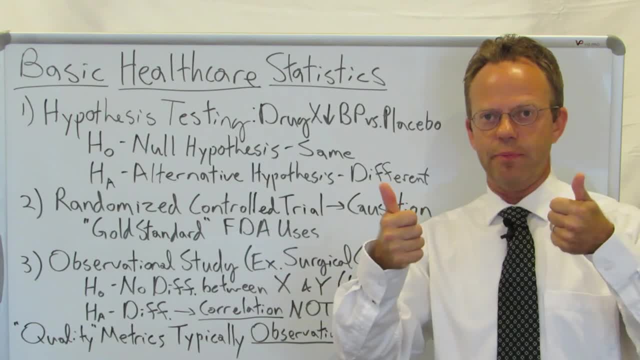 like: oh, that's not going to work, It's only a sugar pill, And so that raises your blood pressure. And so you might say: oh well, look, the blood pressure pill works versus the placebo, because the people taking the placebo were stressed. 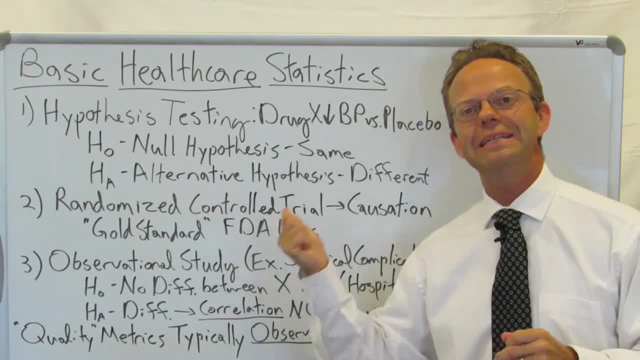 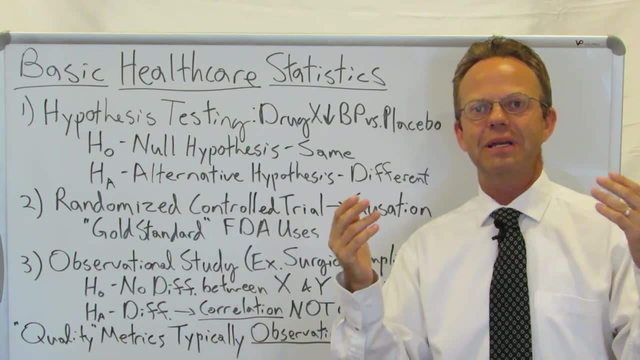 Okay, so that's why it has to be blinded. And then it even has to be blinded to the researchers themselves When they're analyzing the data. they can't know which group had the placebo versus the blood pressure pill, because the researchers themselves will subconsciously 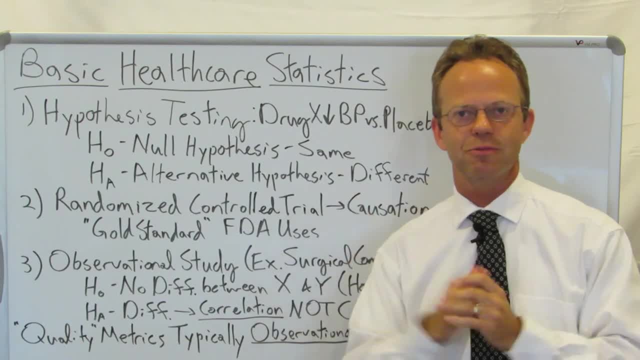 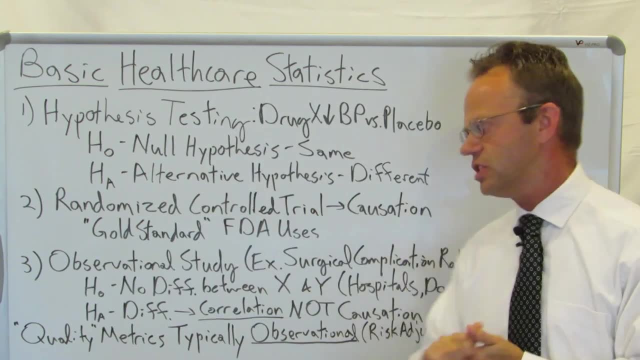 or consciously bias their analysis of the data to give them the results they want. Okay, fine, What's another way to generate data? It's referred to as an observational study, right, And so this is where you know we might observe a surgical complication rate. 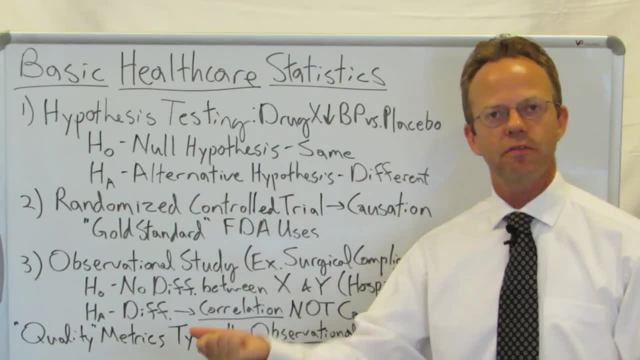 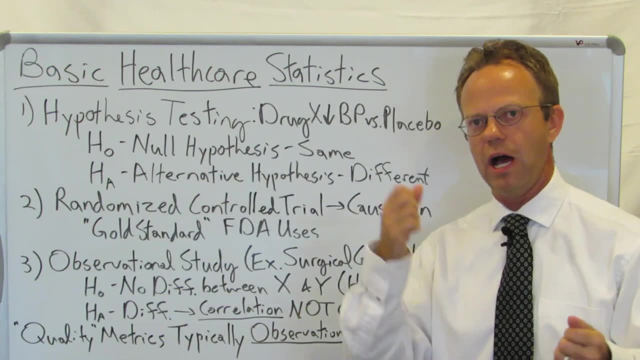 at one hospital. Okay, so this is where you might observe a surgical complication rate at one hospital versus another, or for one surgeon versus another. Again, you can have a null hypothesis which says there's no difference between X and Y, no difference between one hospital or another, no difference between 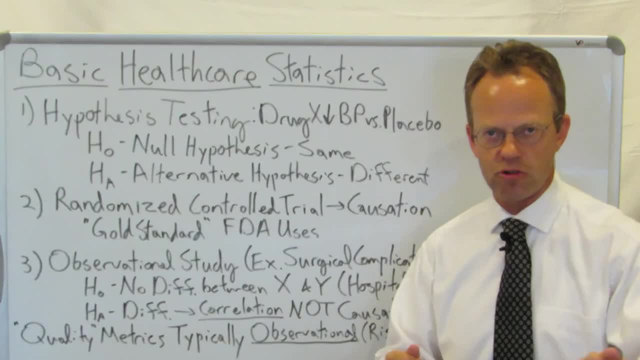 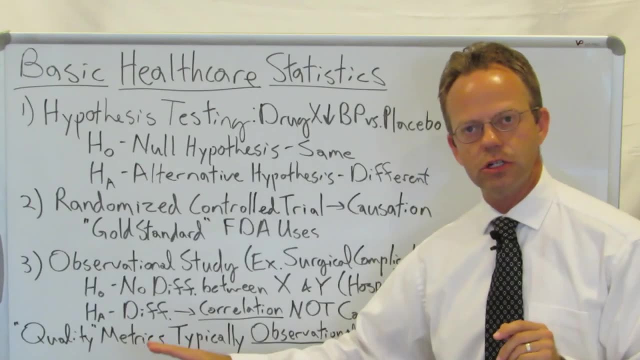 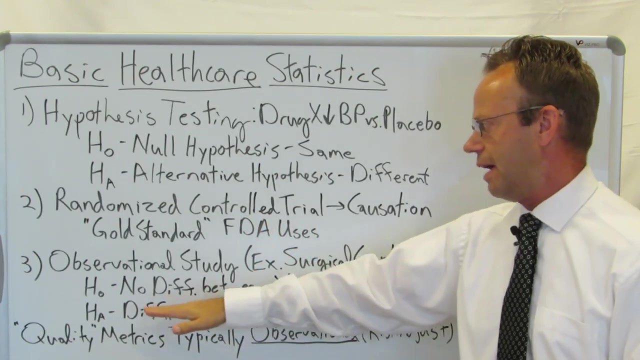 one surgeon or another, no difference between one state or metro area and another. And then there's the alternative hypothesis that there is a difference. Okay, now in an observational study, because it is not randomized, right, You don't randomize the people that went to one hospital. 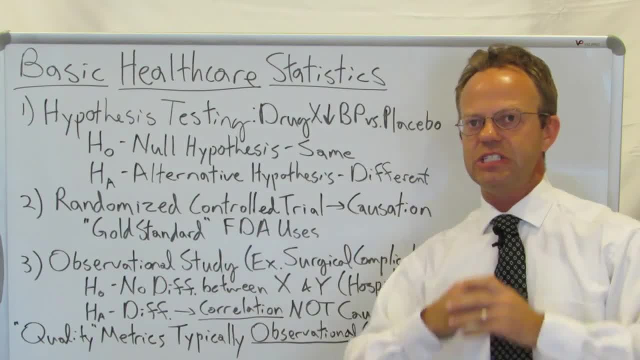 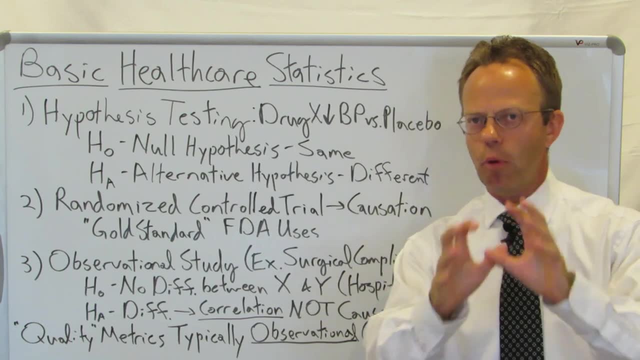 or another, or that went to one surgeon or another. because it's life, It just kind of happened on its own. Okay, so, because we cannot prospectively randomize it. what that means is- and this is the point I'm making- 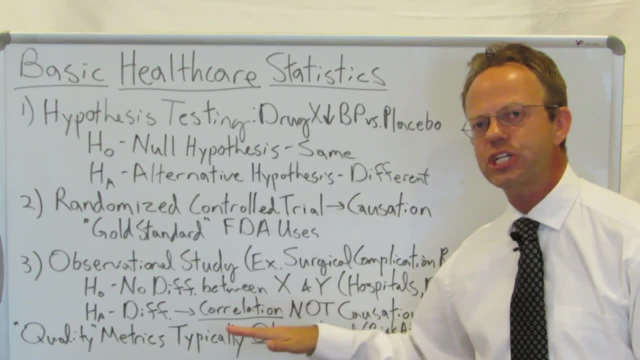 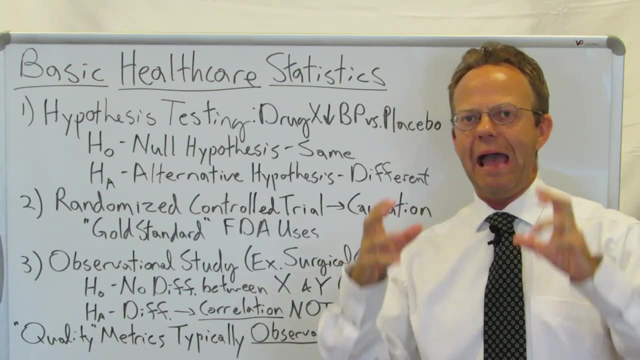 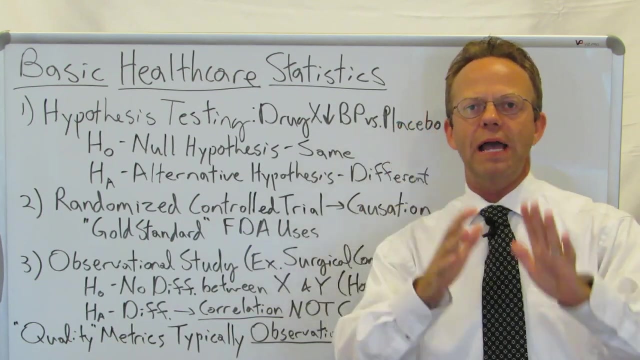 with this video is that an observational study only proves correlation, not causation. It's the whole rooster crowing and the sun rising thing right, The two of them happen together, but it doesn't mean that the rooster crowing caused the sun to rise. Okay, Now why is this specifically?